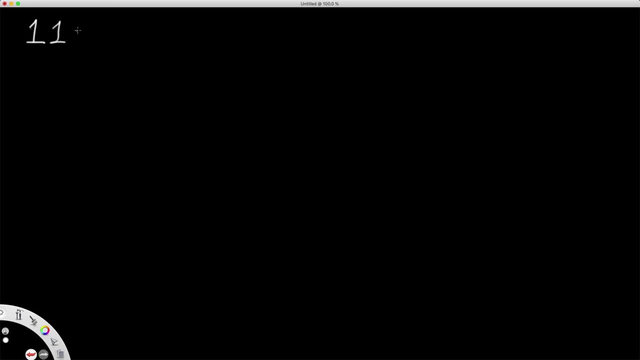 here is going to consist of all 1s, right? So 1, it could be, whatever it is, it just has all 1s. So, keeping that in mind, we know for a fact that it is going to end the value 1, right, And we know 1 is odd. So now let's just look at our k values. So, for whatever, 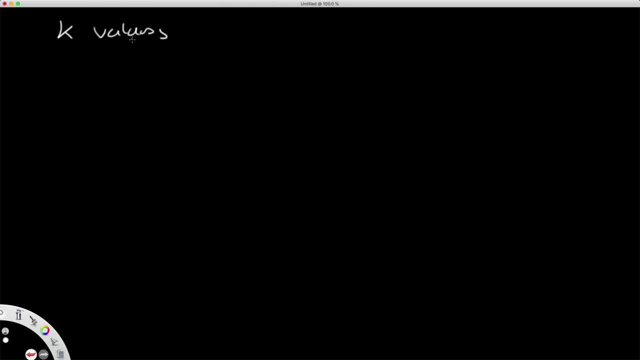 possibility, whatever possibility of values we have for k, they are always going to end in the number 0,, 1,, 2,, 3,, 4,, 5,, 6,, 7,, 8, or 9, right? So that's pretty obvious. Obviously, all numbers. 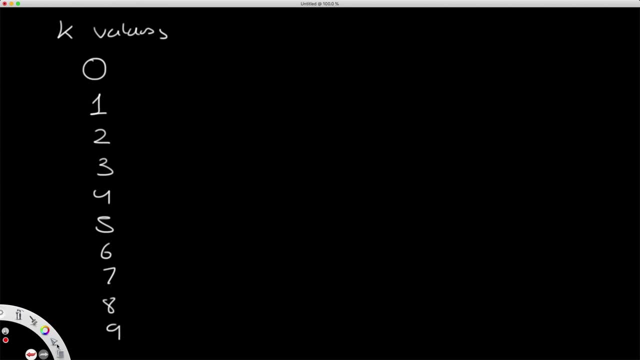 end in 0 through 9, right? So in this case we can actually make our question a little bit easier. So let's just look at the even numbers in the beginning. So we have 0,, we have 2,, 4,, 6, and 8,. 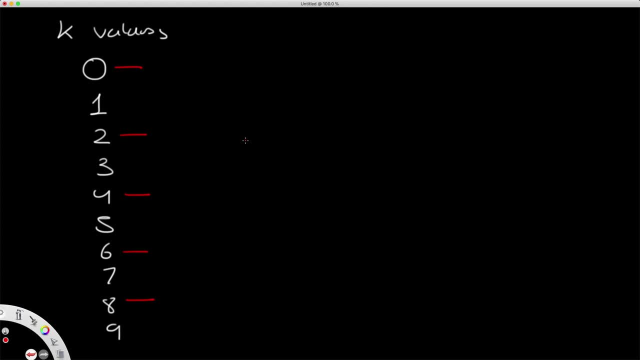 right? So whenever a number ends with an even number, all of its multiples are going to be even. So let me just write it down. Okay, so the multiples of even numbers are always going to be even, And that actually tells us that we are never going to have some sort of multiple. 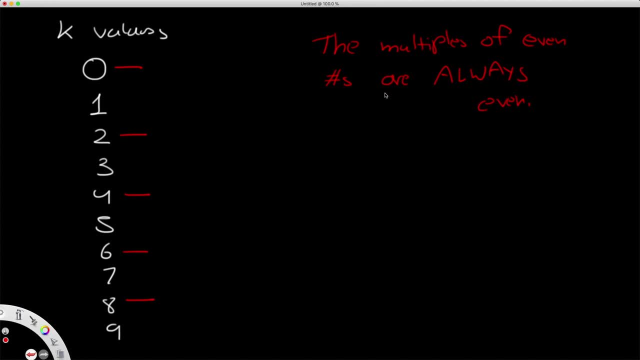 which ends with the value 1.. So what we can do is we can directly eliminate the value whose unit place value or the starting value starts with any of the odd numbers, right, So sorry, even numbers. So if it's 0,, 2,, 4,, 6, or 8, we are never going to find an answer. 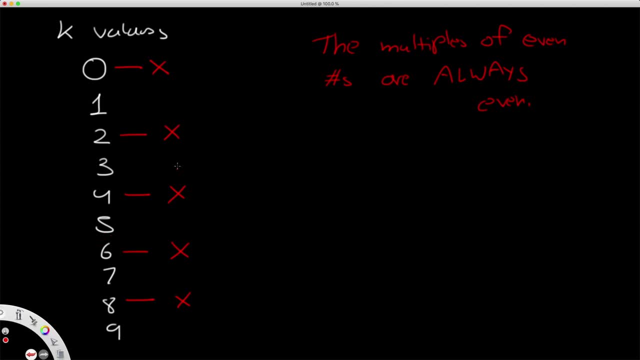 and we will directly just return negative 1.. Okay, so this kind of clears it all up. Now let's just look at the other possibilities. So in this case we have the number 1.. So if we have the number 1 as a k value, or any k value ending with the number 1, or in the units place, 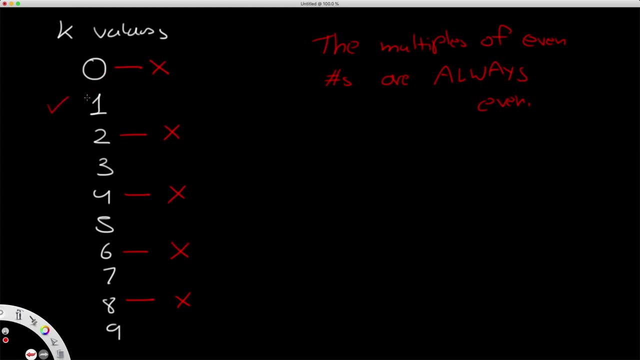 in that case we can find a possible answer. So this is a possibility. So any k value ending with 3 is also a possibility, but any k value ending in 5 is not a possibility. So why exactly is that? So all multiples of whatever number which is ending with 5 is either going to be 0- 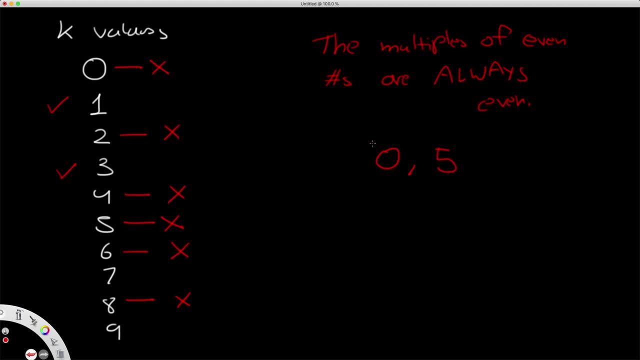 or 5, right, You can look at the multiples. They're always going to end in either 0 or 5.. There's no other option. But we're looking for something which ends with the value 1, because all the numbers inside of n are going to be 1.. So this over here is also not going to be. 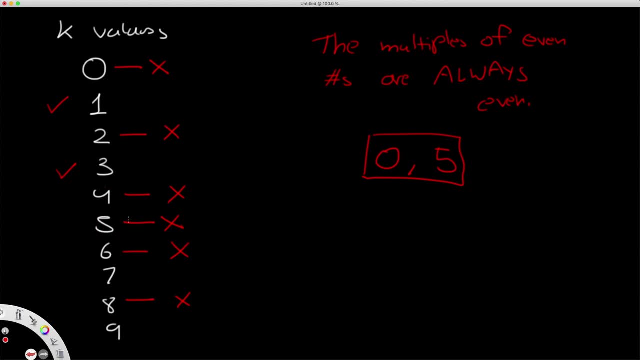 a valid solution. So whenever we have a k value which starts or ends with 5, then in that case we can just eliminate that. Okay, and one more thing I just want to be clear. I keep mixing up between starts and ends. This over here refers to whatever is at the unit place. okay. 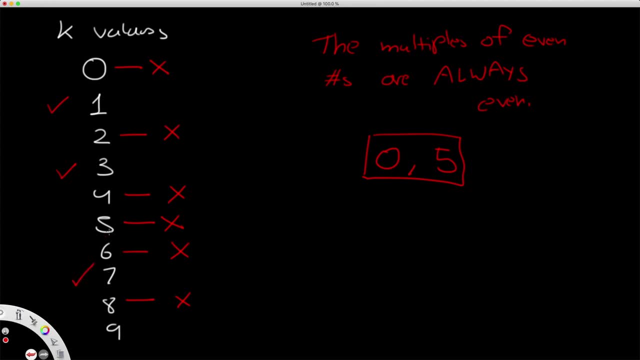 Then 7, if 7 is in the unit place, that could also be a possible answer, and same for 9.. So this over here can be one sort of way that we can get our solution. So we're first going to check if whatever is in the unit's place is not 0,, 2,, 4,, 5,, 6, or 8.. 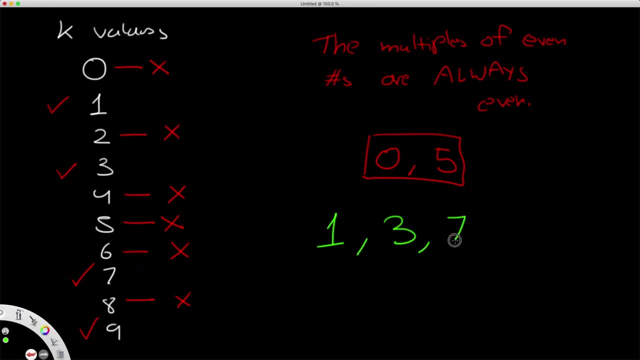 We're looking for something which is either 1,, 3,, 7, or 9.. If anything has 1,, 3,, 7, or 9 in the unit's place, then we know that we have a valid answer over here And in that case we are going to go. 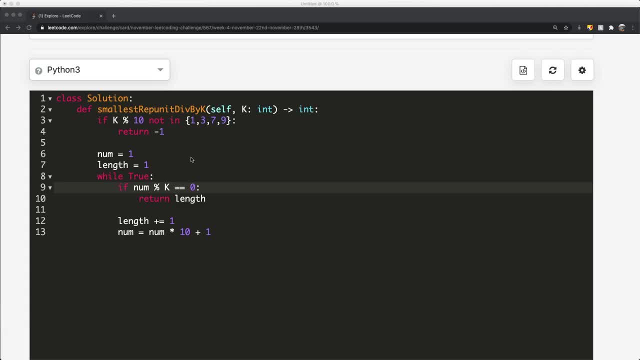 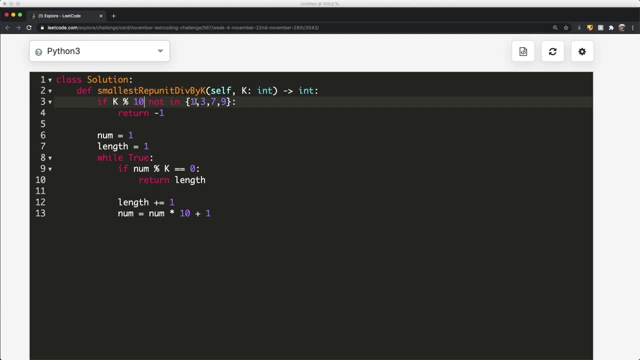 in some sort of while loop, for example, and find the answer. Okay, so this is the code that I wrote. I'll just go through it real quickly. So over here we're checking if whatever is in the unit's place is not in 1,, 3,, 7, or 9.. Then in that case, 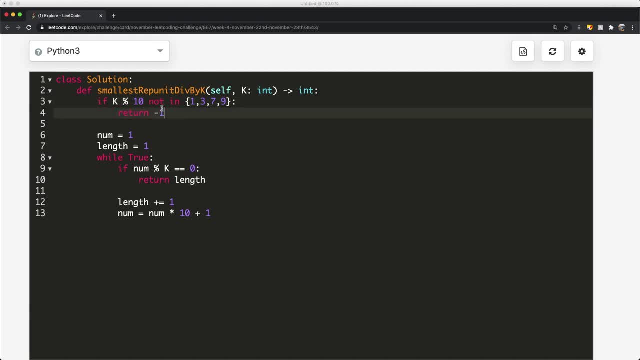 we're directly just returning negative 1, because we're never going to get an answer. So after that we have the number, So the number over here is going to be the end value, and we have a length, and which the length starts off 1,. right, Because the number is 1,. 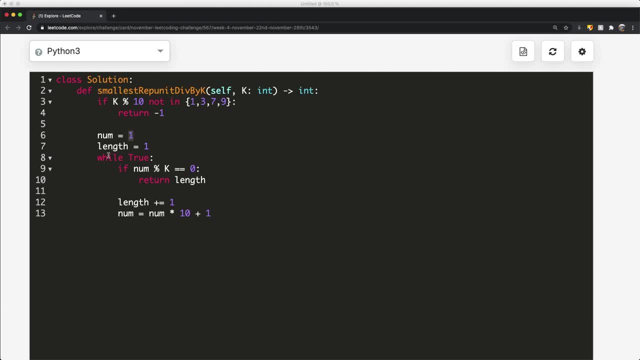 and the number 1 has a length of 1.. So what we're going to do, we're going to go inside of a while true statement, And if the number mod k is equal to 0, then in that case we're going to return whatever length we are at, And if that is not the case, we're going to add an. 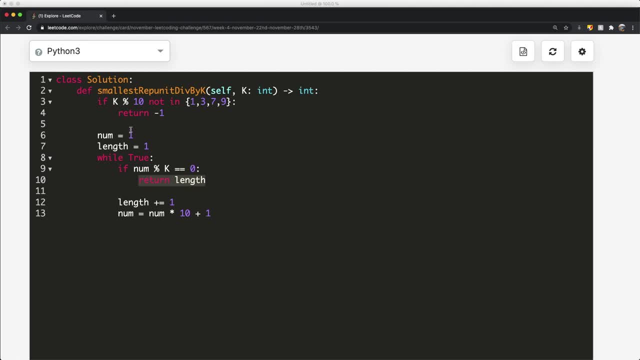 extra 1 to our number. So in the beginning our number is 1.. So now the next value is going to be 11.. So to get that, we do 1 into 10,, so 10, and then plus 1,, giving us a number of 11,, right? So? 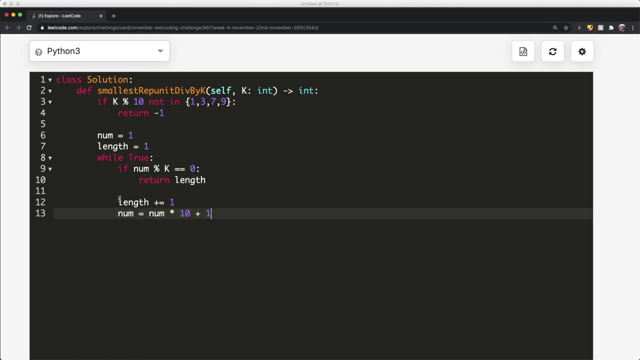 we're going to update our number like that, And each time we're also going to increase the length by 1.. Okay, so that should be it for our solution. So, as you can see, it did get accepted, So yeah.